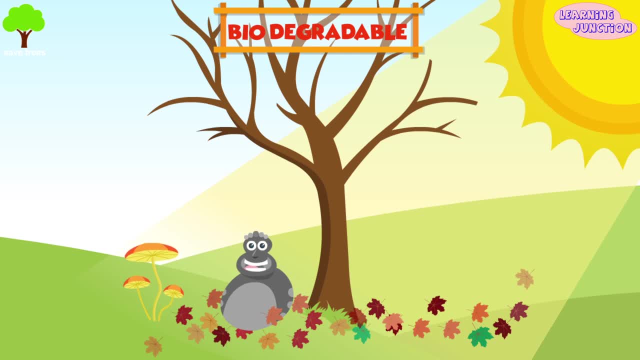 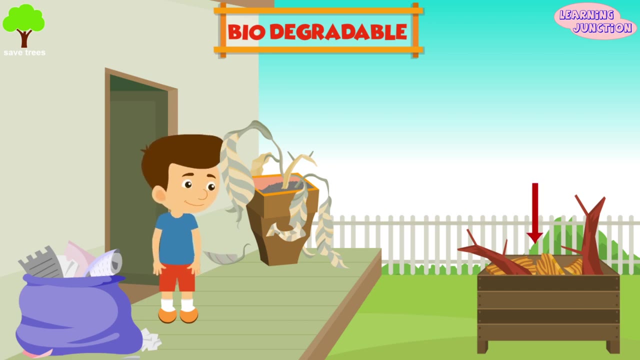 The whole process is natural, which can be slow or rapid depending on the object. Therefore, the environmental risks and issues caused by biodegradable wastes are low. Some biodegradable wastes are paper waste, dead plants, wood, etc. Now the non-biodegradable waste. 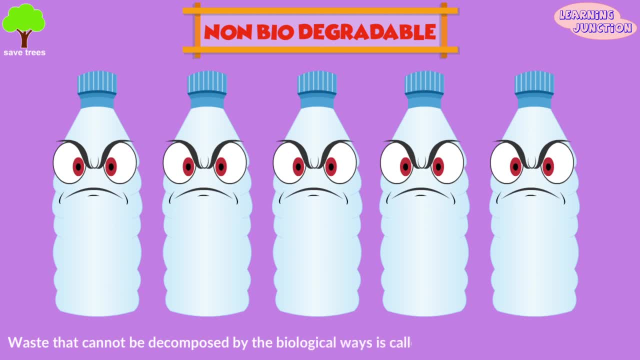 wastes that can be broken down by microorganisms or decomposers and not be adding to any type of pollution. wastes that can be broken down by microorganisms or decomposers and not be adding to any type of pollution. The material that cannot be decomposed by the biological wastes is called the non-biodegradable waste. 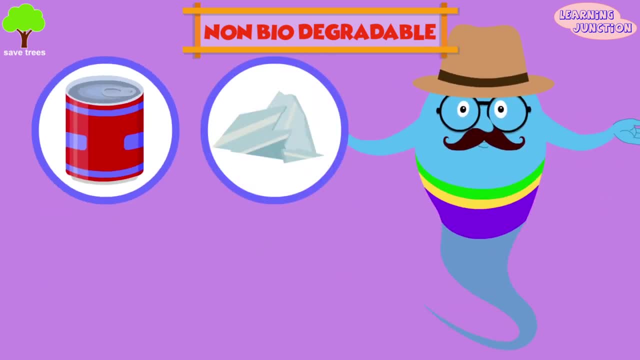 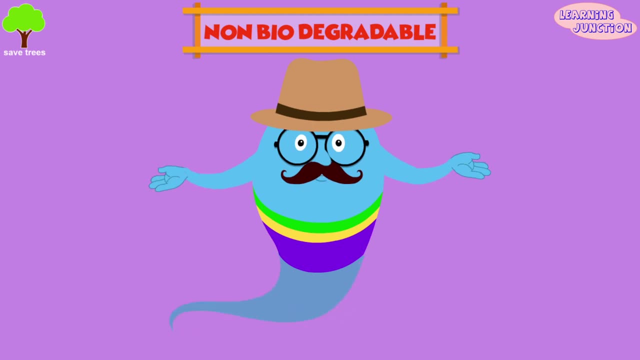 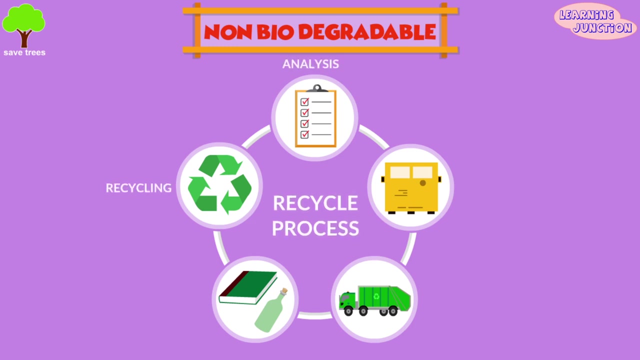 Most of the inorganic wastes, like aluminum cans, glasses and plastics, are non-biodegradable. This can be further classified into recyclable and non-recyclable waste. Here's the process of recycling the waste At first: recycling, analysis, collection, transportation and recovery. 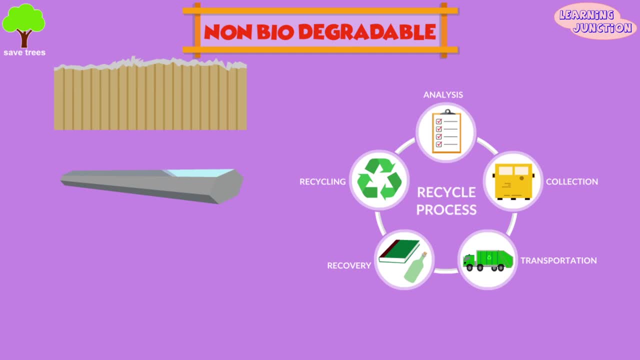 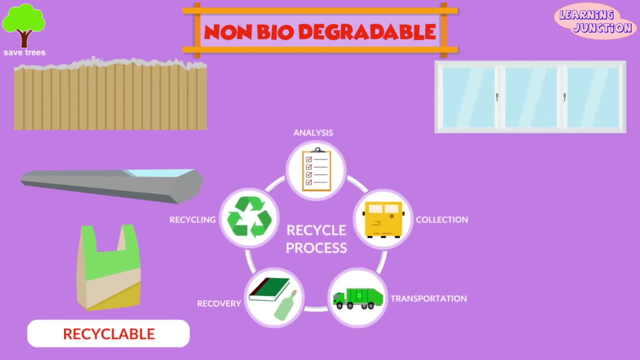 Non-biodegradable waste, such as cardboard, metal and some grocery bags can be recycled, are called the recyclable waste. Some wastes, like fiberglass, kitchenware, auto parts, etc. which cannot be recycled, are called the non-recyclable waste. 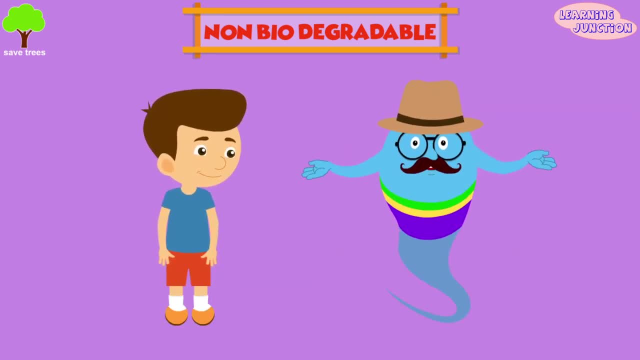 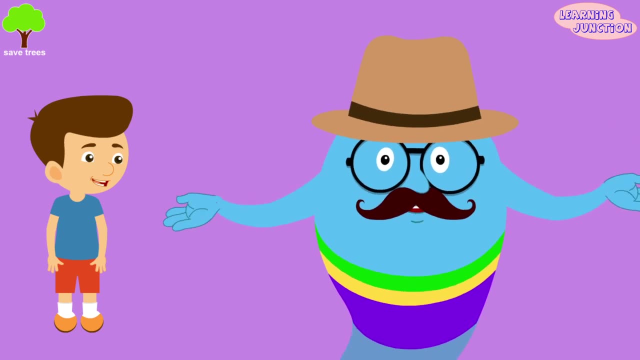 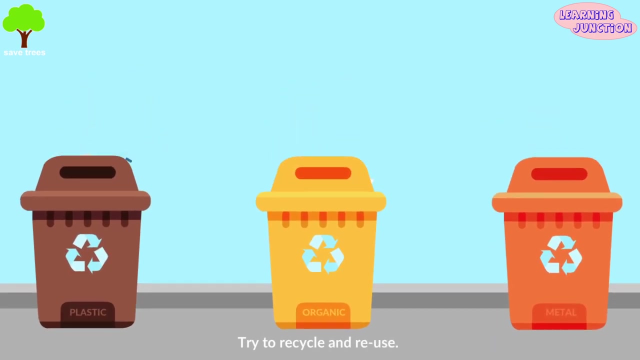 Since non-biodegradable wastes are not environmentally friendly, they need to be substituted. Waste is harm for everyone. Guys, here is some simple ways to reduce waste. Try to recycle and reuse. Do not use plastic bags. Use paper, jute or cloth bags. 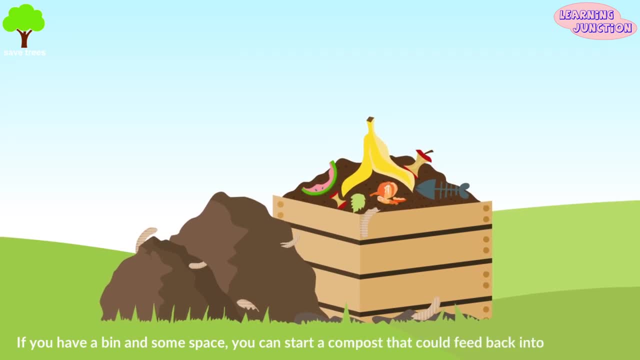 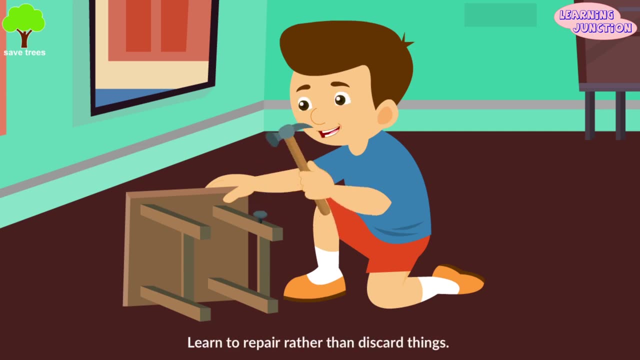 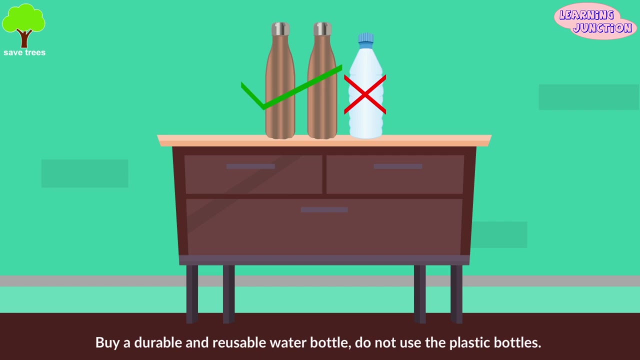 If you have a bin and some space, you can start a compost that could feed back into the garden. Learn to repair rather than discard things. You're doing great buddy. Buy a durable and reusable water bottle. Do not use the plastic bottles. 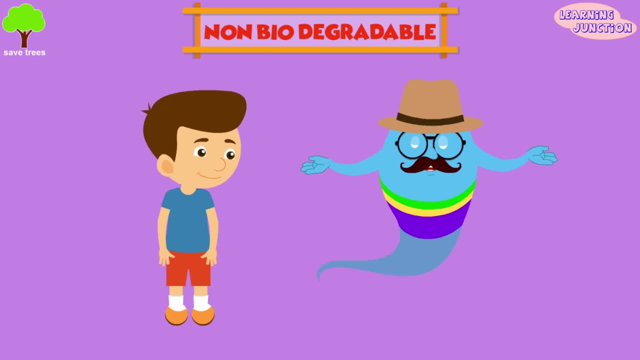 Now you know a lot about biodegradable and non-biodegradable wastes. Stay tuned for more videos. Bye-bye.